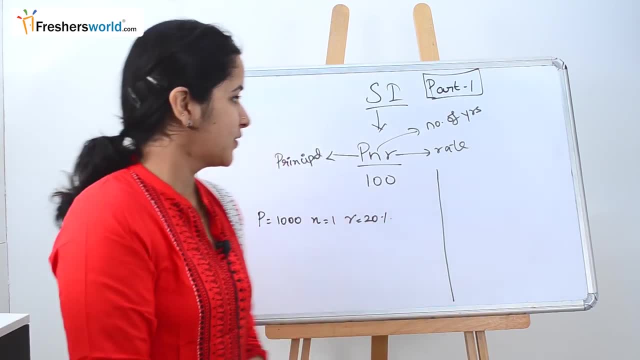 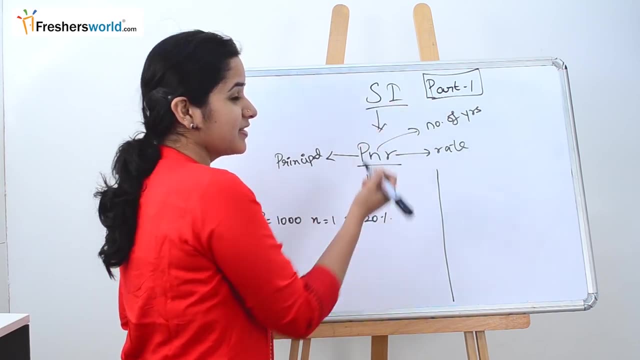 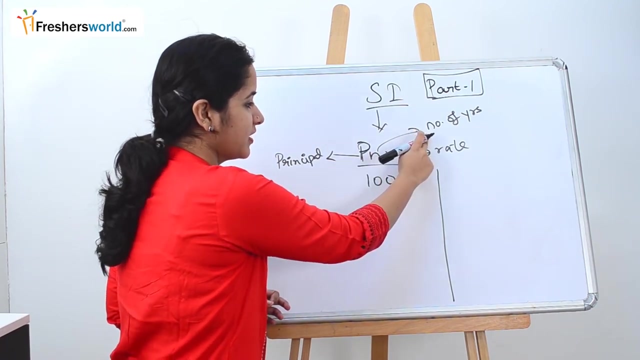 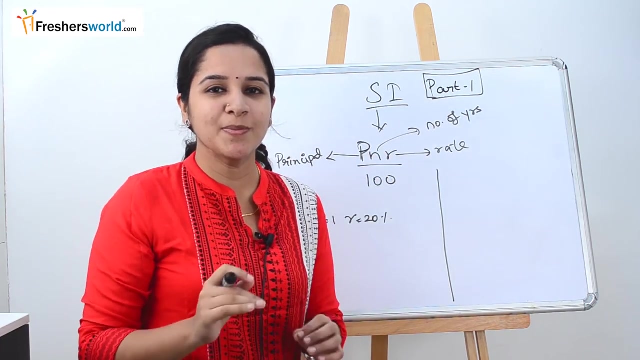 The topic that we are going to look today is simple interest. So in order to solve the sums in simple interest, there is just only one formula you need to know, which is nothing but simple. interest is equal to P and R by 100. So what is P here? So P is nothing but principle. N is the number of years and R is the rate and divided by 100. So you should know this formula to find the simple interest. So what is basically a simple interest? So let's say you are going to put rupees, 1000 rupees, in a bank and then you are going to keep. 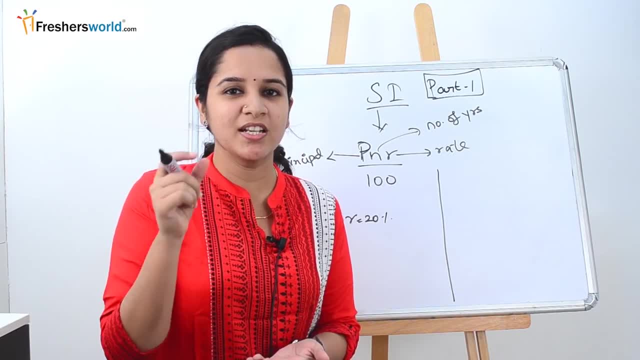 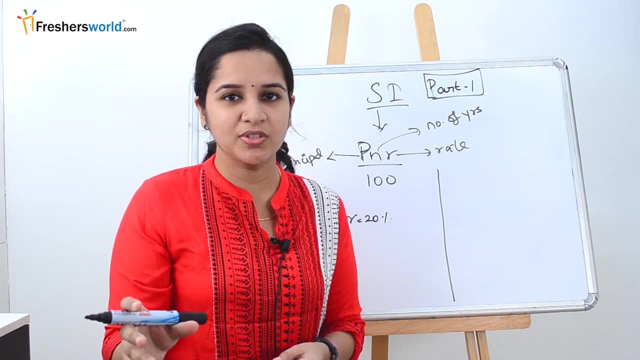 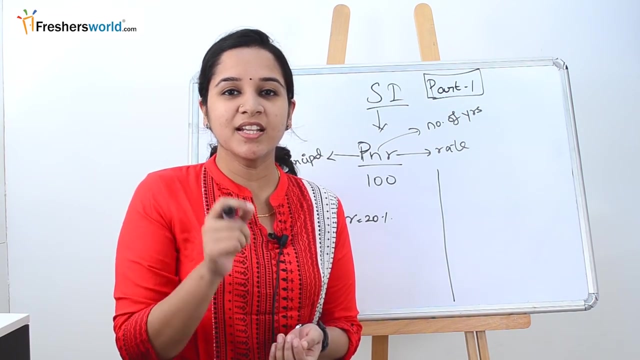 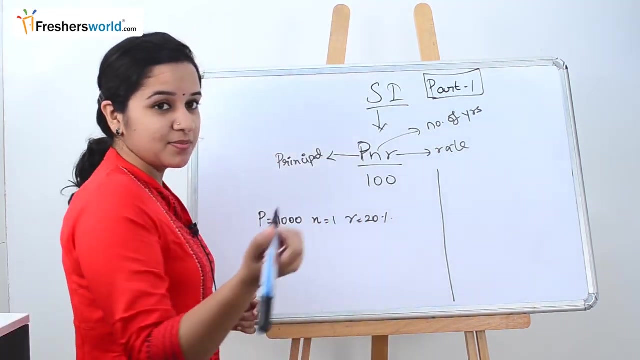 it for 2-3 years, then the interest will be same for each and every year at the end of the year. So that is the difference between the simple interest and the compound interest. In case of the compound interest, what do you do is that, whatever the interest that you get accumulated at the end of the year plus the amount will be taken for the next year, Whereas in case of the simple interest, the same principle amount that you consider will be there for each and every year. So let's take a small example. Let's say you are going to put 1000 rupees in a bank for a year at a rate of 20%. Now you 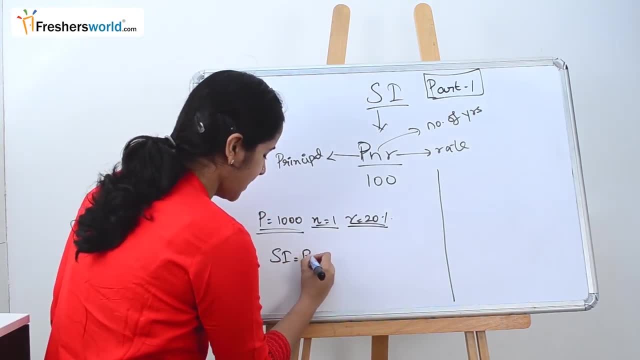 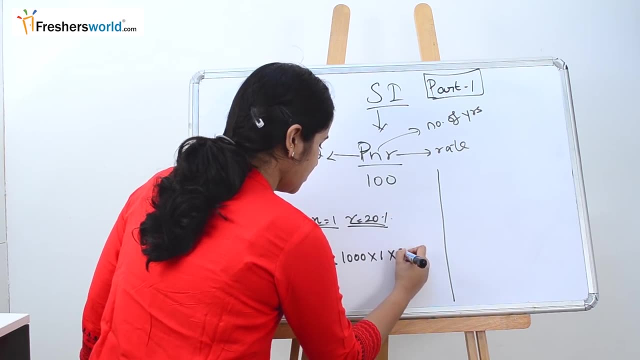 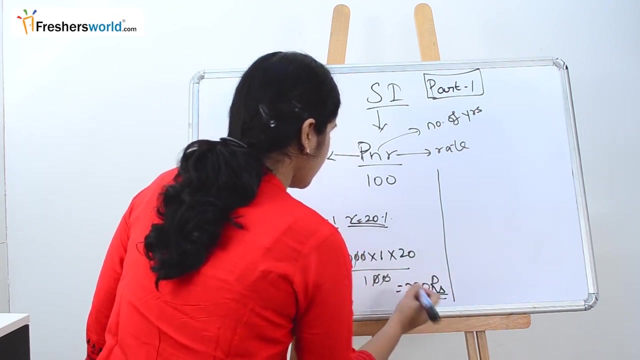 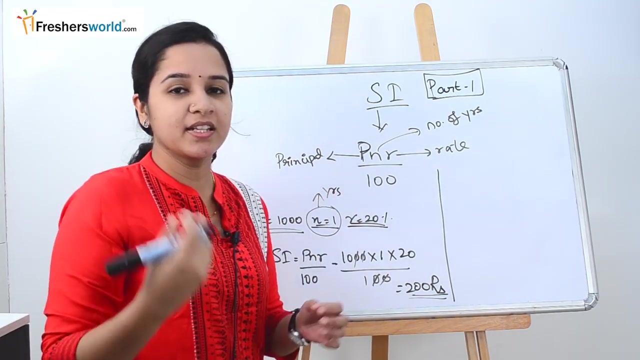 are going to find the simple interest. So simple interest is nothing but P and R by 100. So principle is 1000 rupees, number of years is 1, rate is 20 divided by 100, nothing but 200 rupees. So the interest at the end of the year is nothing but 200 rupees, Always N. if you see it will be represented in years, Let's say in a sum they are going to give you as 9 months. then in that case how you have to represent it is 9 by 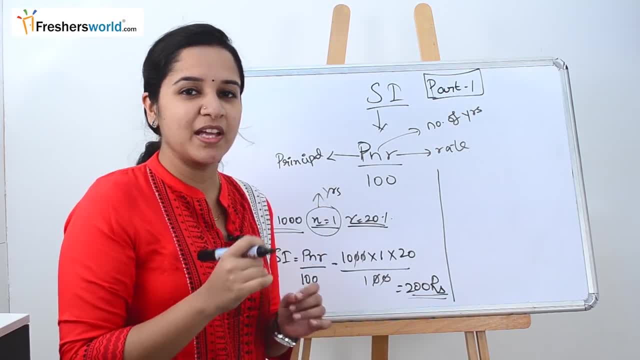 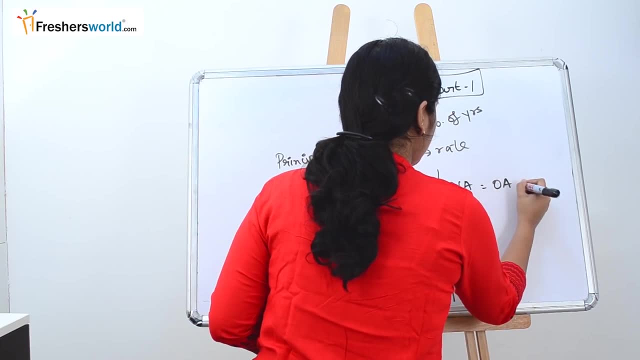 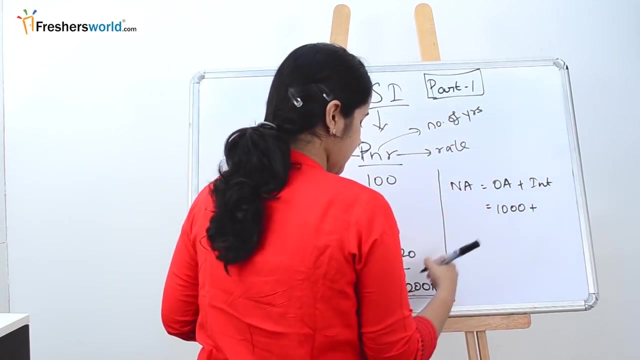 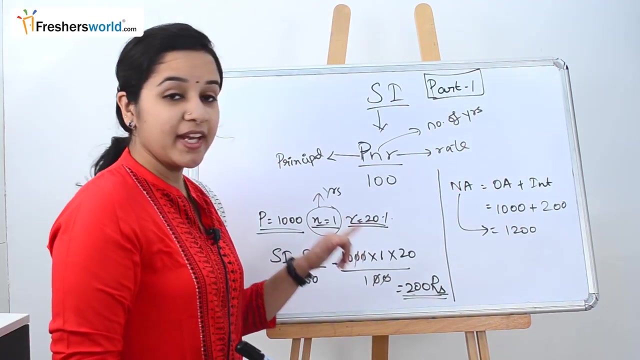 12. So always remember N will be in years. This is where the lot of people make mistakes. Another thing is that so new amount is equal to old amount plus interest. So old amount is nothing but 1000 rupees plus your interest is 200. So at the end, so new amount is equal to 1200.. So at the end of one year you will have the amount as 1200.. How you will get So you have initial. 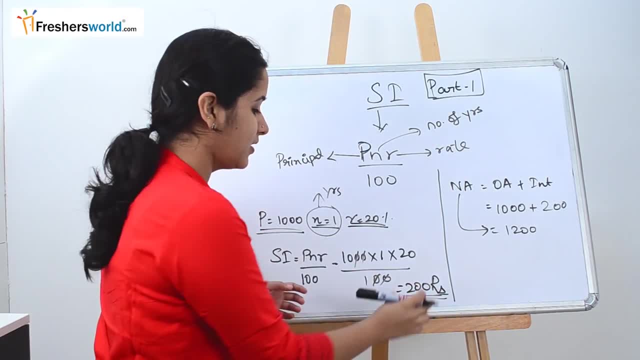 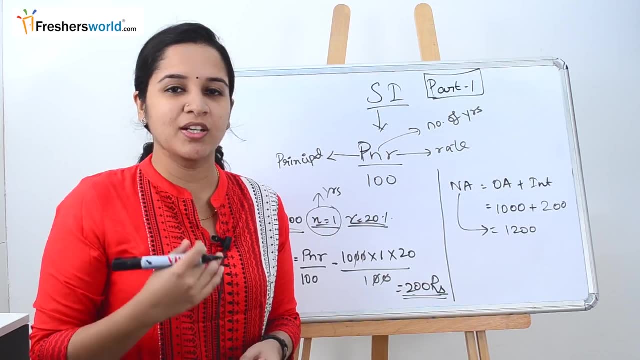 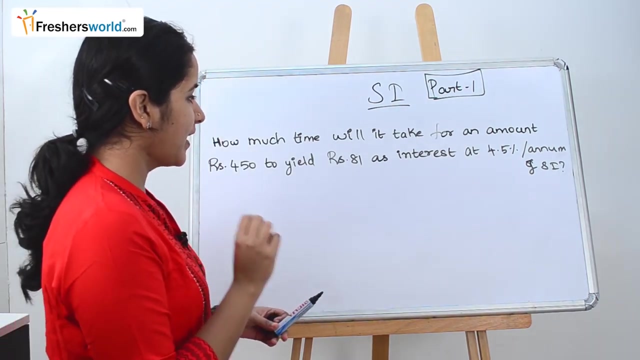 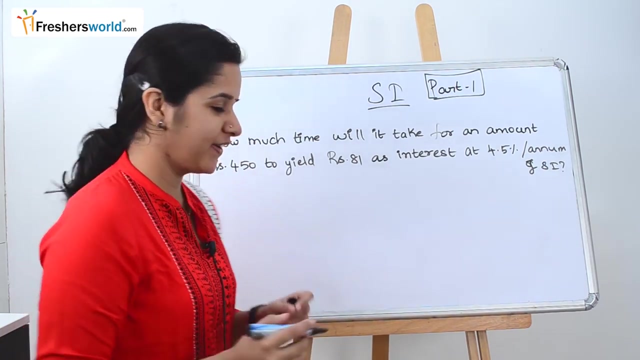 put 1000 rupees in a bank, At the end of one year you are getting an interest of 200 rupees. So together is 1000 plus 200, which is 1200.. Let's solve couple of simple sums to understand this concept better. So the first question is: how much time will it take for an amount of rupees 450 to yield rupees 81 as an interest at 4.5 percent per annum of simple interest? So first let's write the given data. So the given data is: they have given 450 to yield rupees 81.. 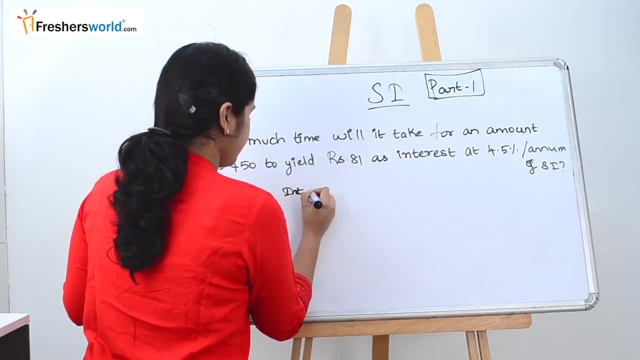 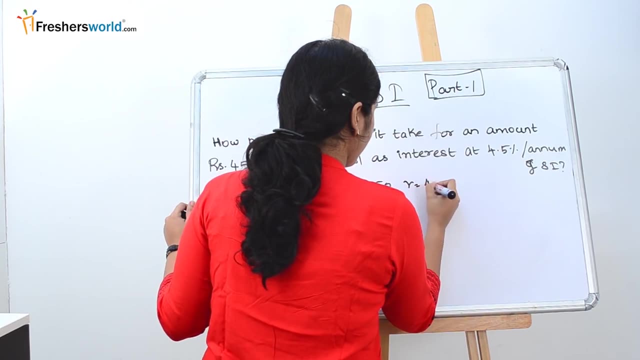 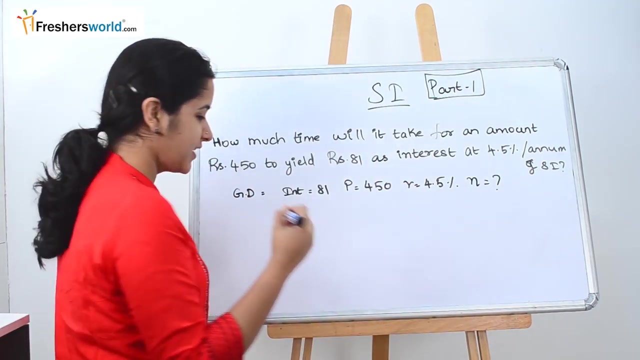 So interest is nothing but 81.. Principal amount is nothing but 450.. At rate, I have given as 4.5%. The question that they have asked is how much time? So they ask us to find the number of years. So how to find it? Let's write the formula. 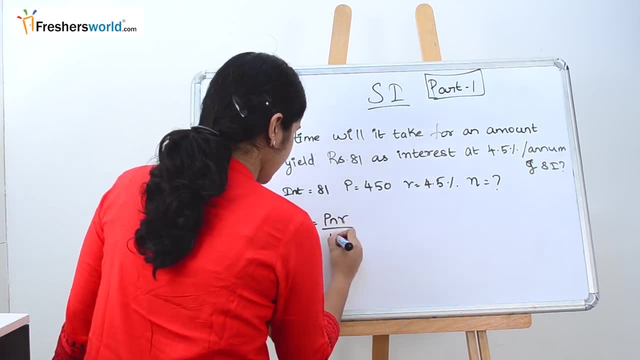 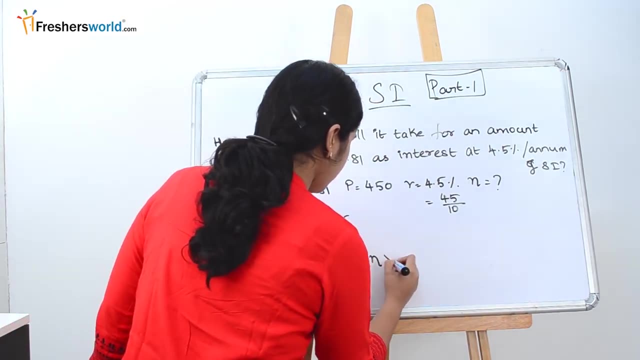 Simple interest is equal to PNR by 100.. So they have given the interest is nothing but 81.. P is nothing but 450.. N, we have to find out, and rate is 4.5, which we can write as 45 by 10.. So already 100 is there, So we can write 45 by 1000. 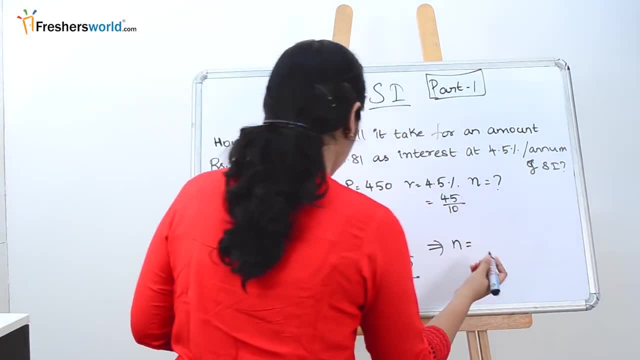 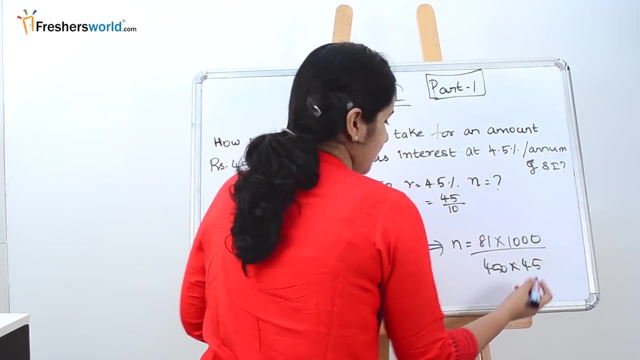 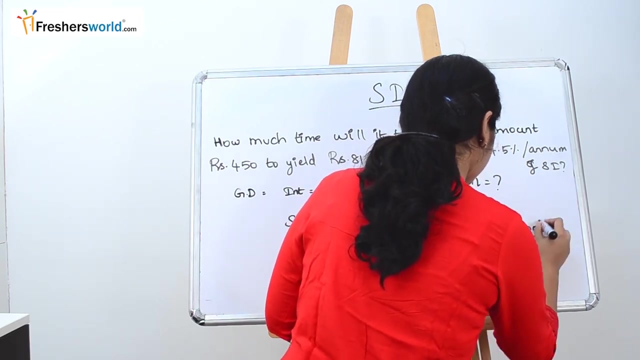 So let's take all everything to one side. So N is equal to 81 into 1000, divided by 450 into 45.. So 9, 5's are, 9's are 200, 9, 5's are, 4's are. So it's nothing but 4 years. 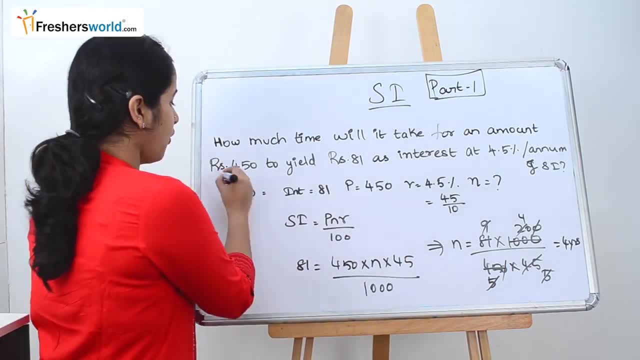 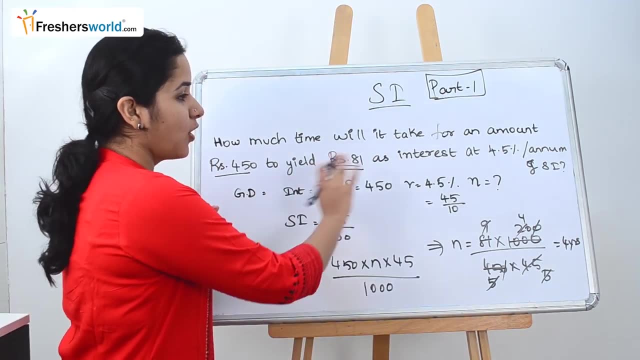 So at the end of 4 years, the amount 450 will yield an interest of 81 rupees at the rate of 4.5%. So how did we do that? We have got all the data. The one that we have to find is N. 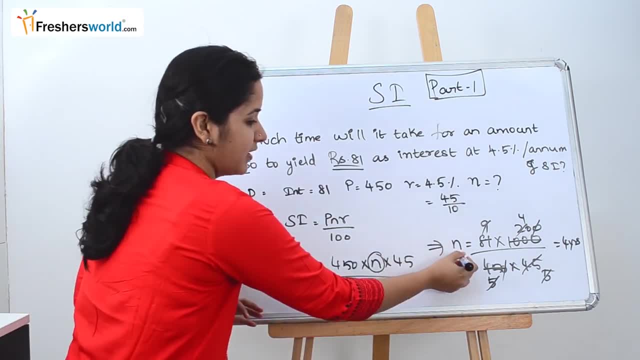 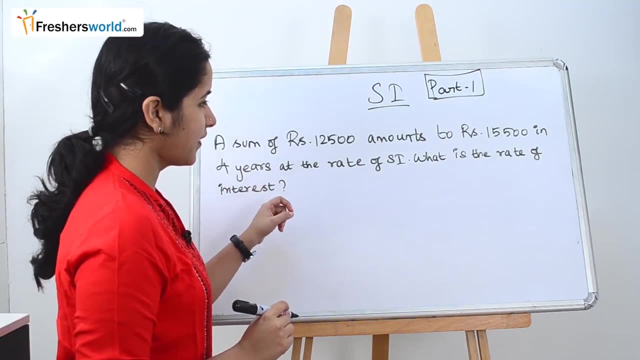 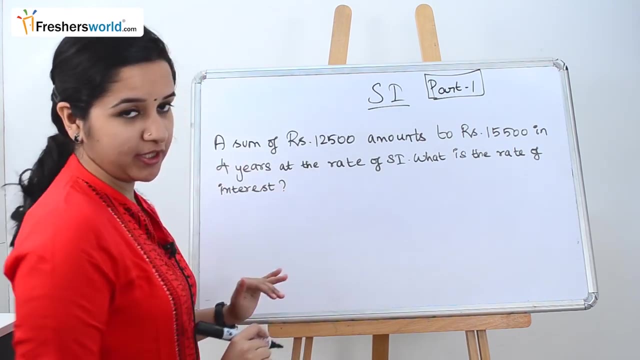 So, whatever the data that we know, we are taking it to one side and finding the unknown. So let's solve another sum to understand this concept better. The next Question that they have given is A sum of rupees 12,500 amounts to rupees 15,500 in 4 years at the rate of a Simple interest. what is the rate of Interest? 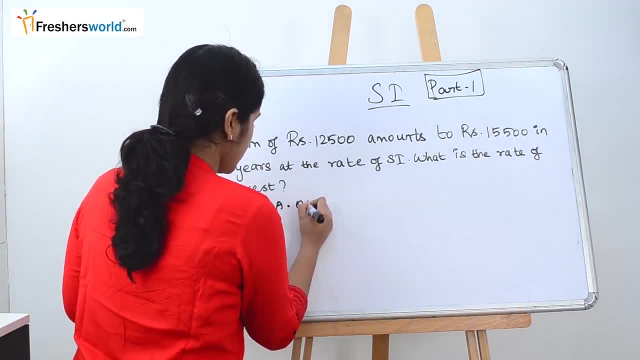 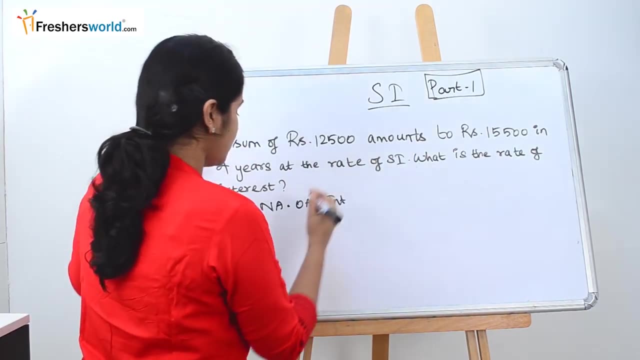 So, as we know that new amount is equal to old amount plus interest, So we know the 12,500 became 15,500 in 4 years. So new amount is 15,500 is equal to this. old amount is nothing but 12,500. 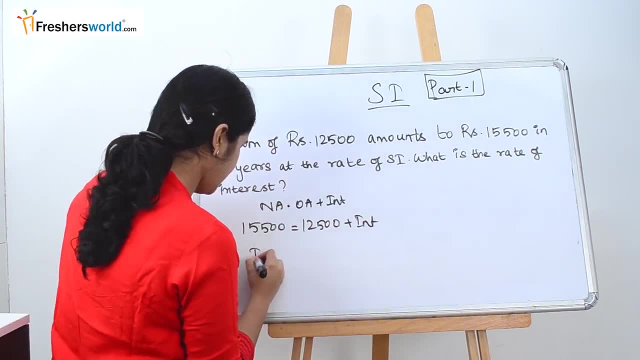 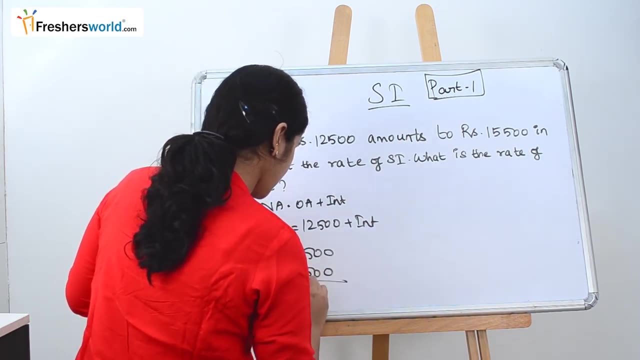 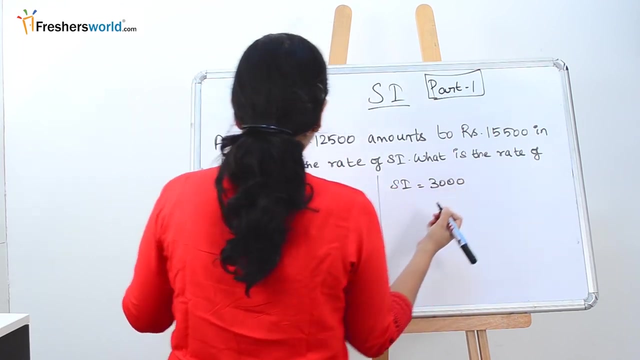 plus the interest. So, in order to find the interest, what do we do? 15,500 minus 12,500, which is nothing but 3,000.. So we know that interest is nothing but 3,000.. The number of 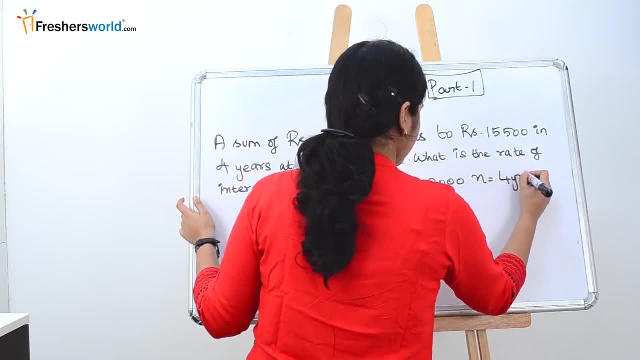 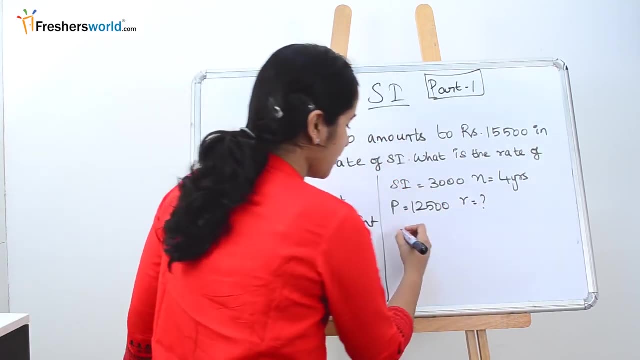 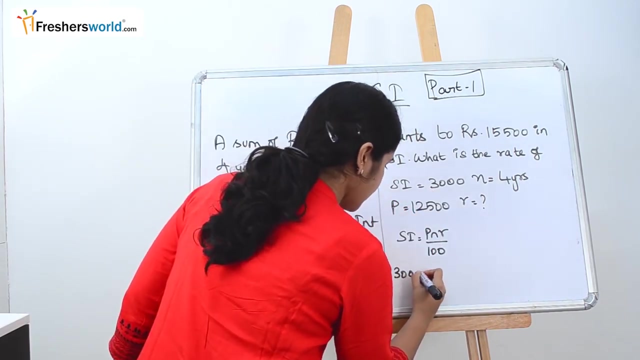 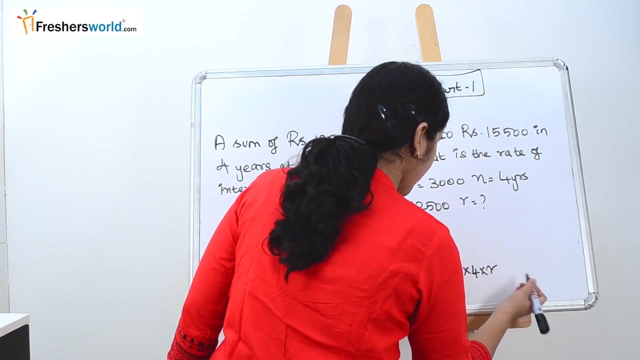 years is nothing but 4 years. We know the principal amount was nothing but 12,500.. Now we have to find the rate Easy, right? So what do you have to do? Simple: interest is equal to P and R by 100.. Interest is 3,000.. Principal is 12,500.. N is 4 years. Rate is the one we have. 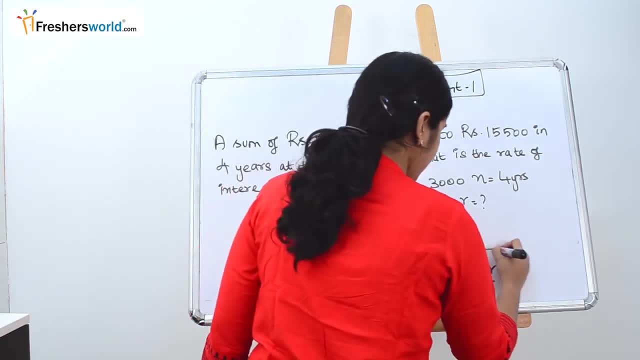 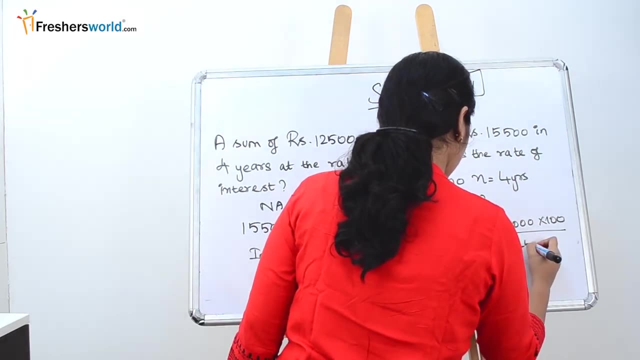 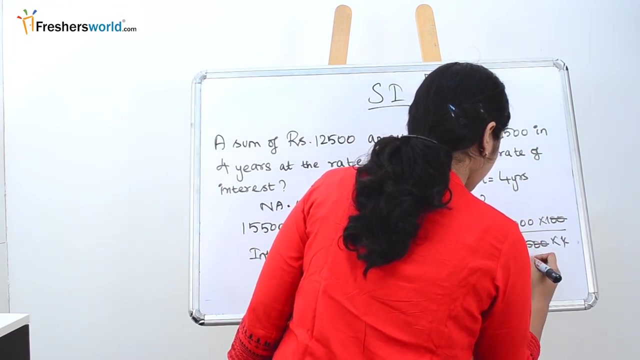 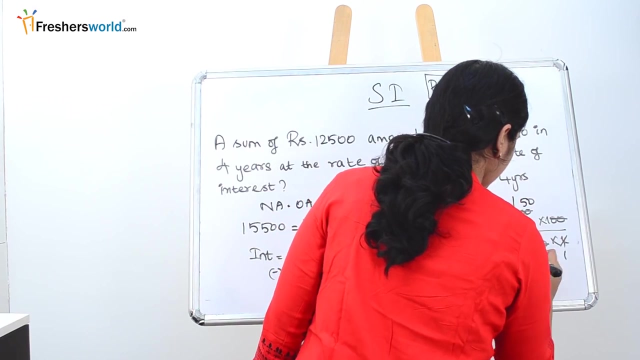 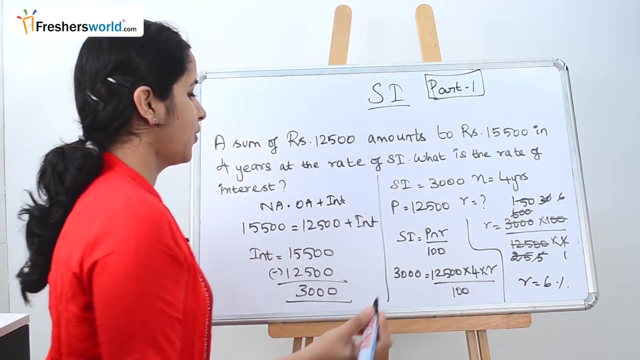 to find, divided by 100.. So take all the unknown to one side. So R is equal to 3,000 into 100, divided by 12,500 into 4.. Cancel: I2s are 25,600.. 1s are 150.. 5s are 36.. So rate is equal to 6%. So at the rate of 6%, 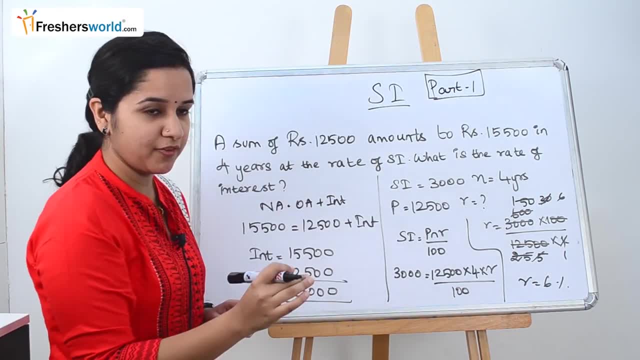 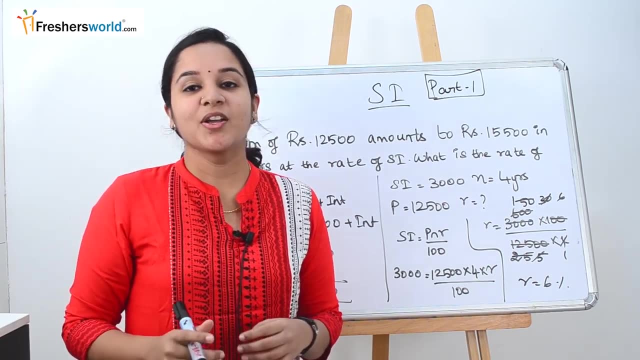 the sum of 12,500 becomes 15,500 in 4 years. Today we got to know the basic concept of simple interest and couple of some of the basic concepts of simple interest. So let's understand the concept better. So in the upcoming videos we will be solving much tougher. 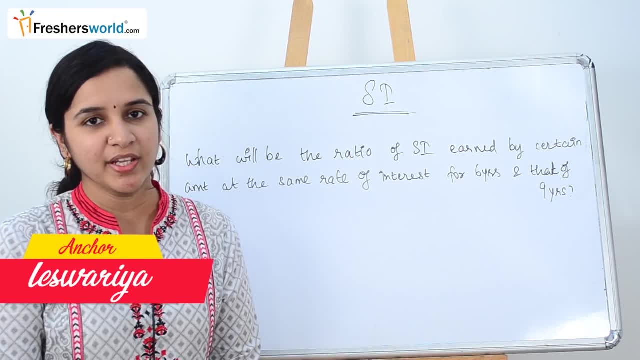 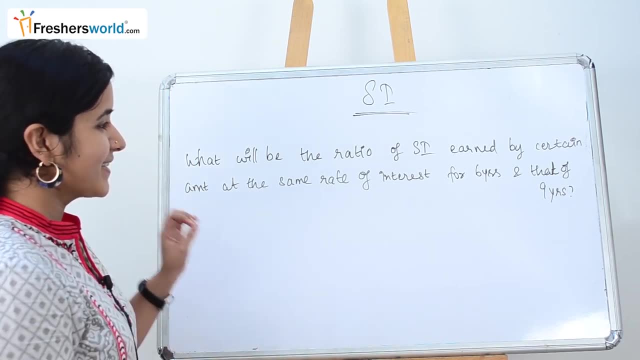 problems to understand this concept much better. The topic that we are going to look today is simple interest. So let's get started. So the question is: what will be the ratio of simple interest earned by certain amount at the same rate of interest for 6 years and that of 9 years? 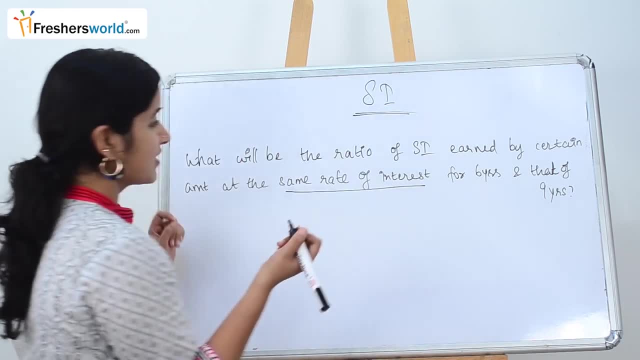 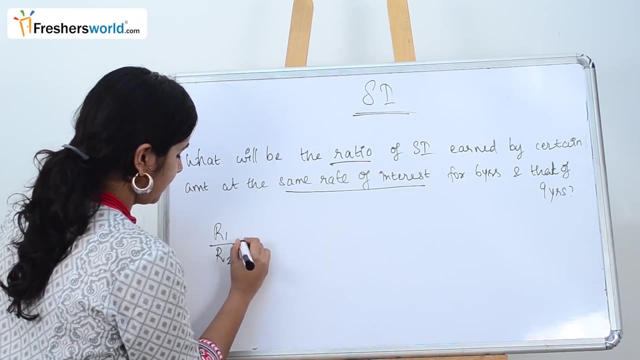 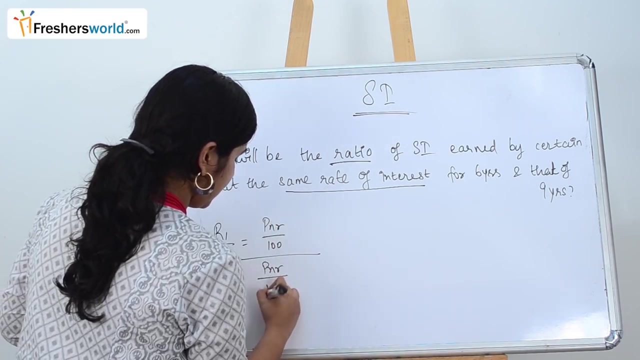 So they have given the same rate of interest, So they are asking you to find the ratio. So for 6 years and 9 years, So ratio 1 divided by ratio 2.. With the simple interest we are going to do, which is nothing but PnR by 100 divided by PnR by 100, for 6 years and 9 years. 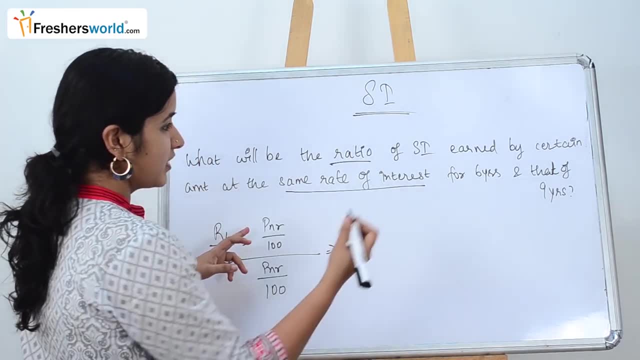 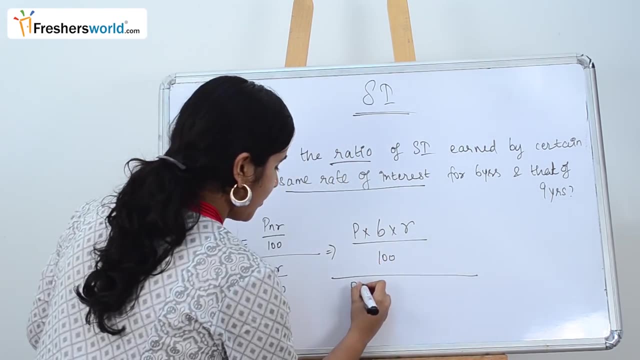 So what is the principal amount? We don't know. What is the number of years? We know it's 6 years Rate is common, So you can take it as R divided by 100, divided by principal, We don't know. 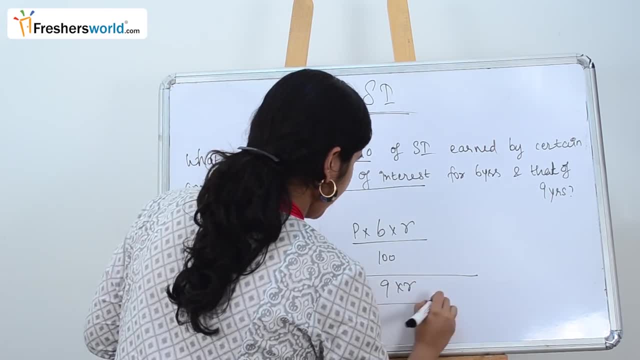 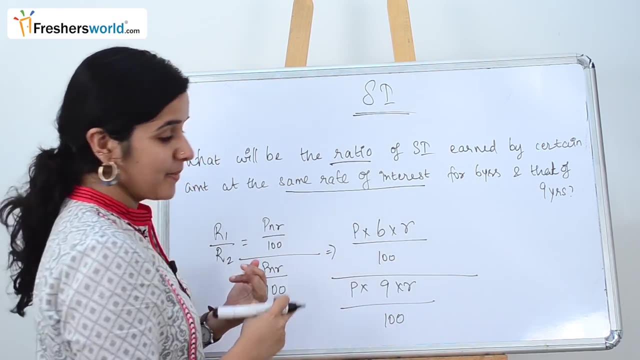 Number of years is 9.. R is same divided by 100.. As we know, the same principal is the one that we are going to take for 6 years and 9 years. We know P is also same and R is also same, So it can be cancelled. 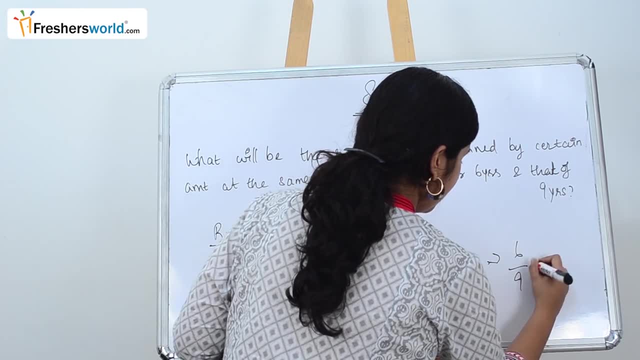 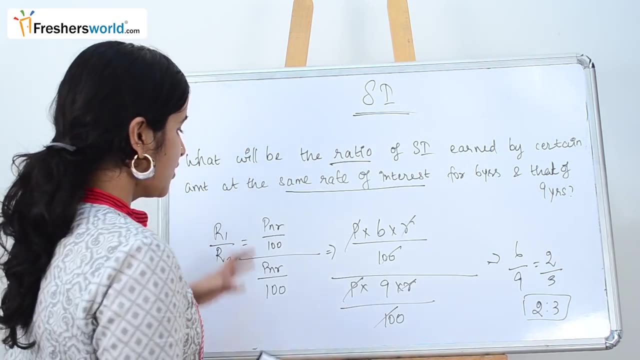 P, R and 100 is also cancelled. So it is nothing but 6 by 9, which is 2 by 3.. So the ratio is nothing but 2 is to 3.. So this is a very simple and a classic problem. So what you have to do is that- though they didn't mention that, 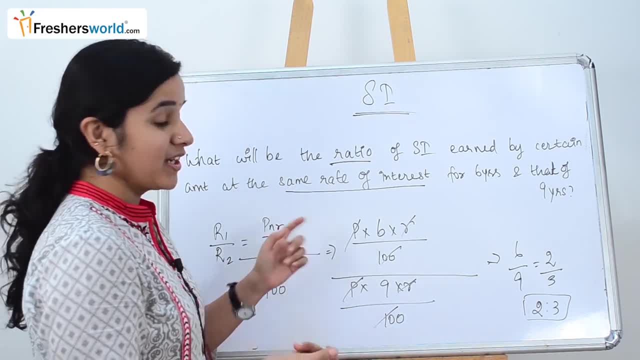 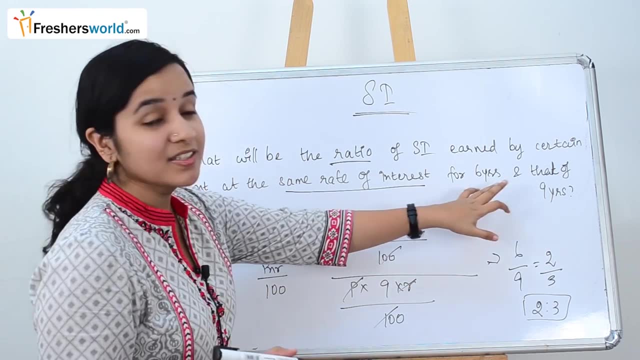 principal is same or not. lot of people get confused whether we have to take it as P1, P2 or something like that, But we know that the simple interest is earned for the same amount for 6 years and the 9 years. 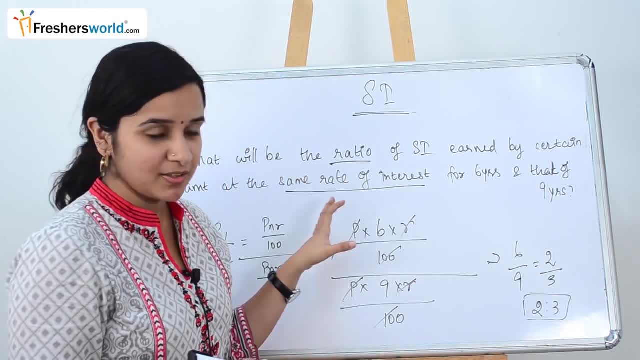 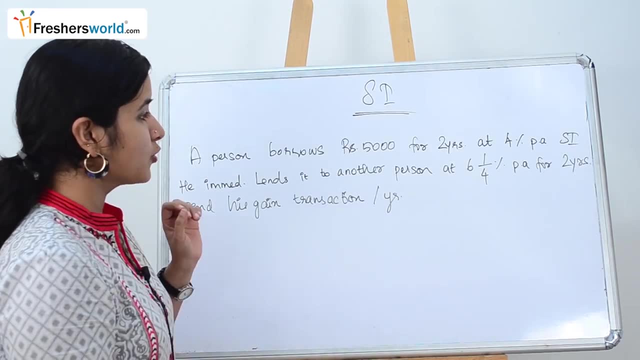 So P will always be the same here, though they didn't mention explicitly in the question. So P and R gets cancelled. So easily you can find the ratio. Let's go to the another sum. So the next question is: a person borrows Rs.5000 for 2 years at 4% per annum, simple interest. 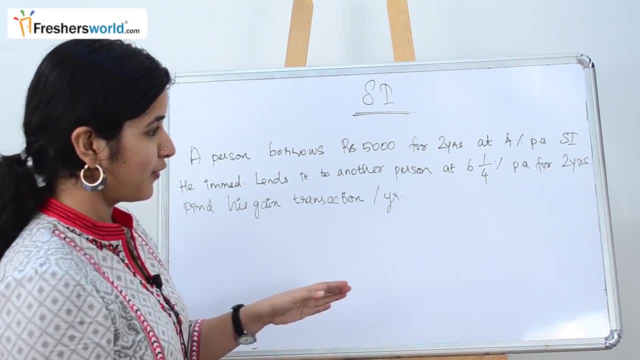 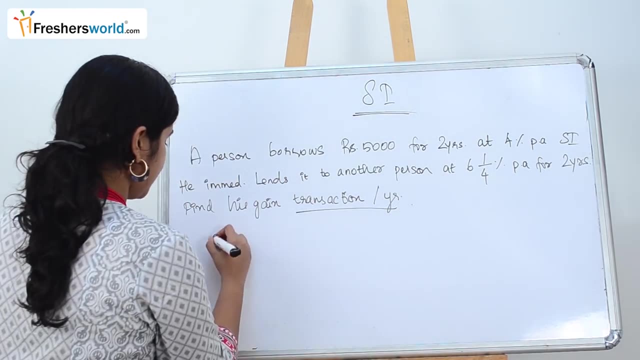 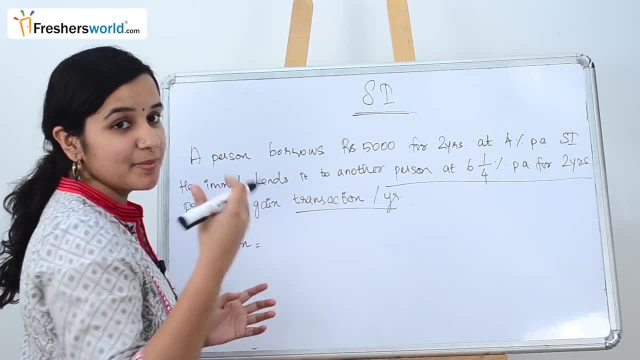 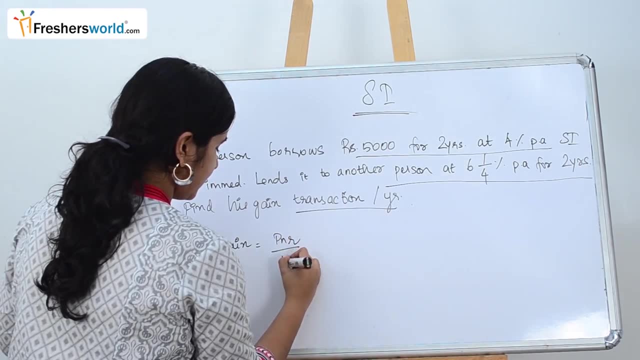 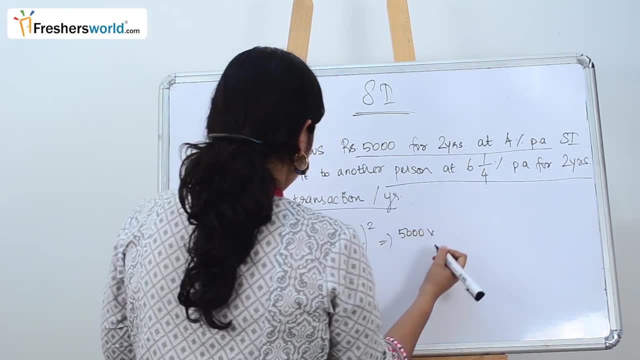 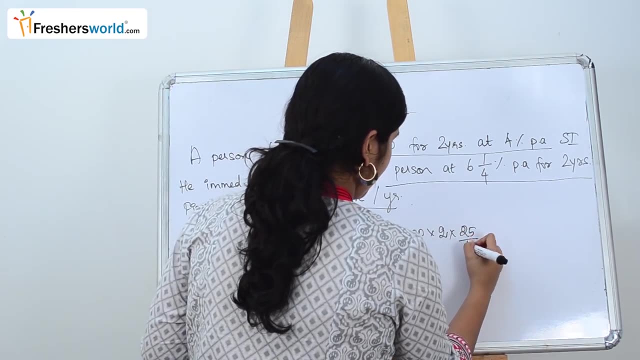 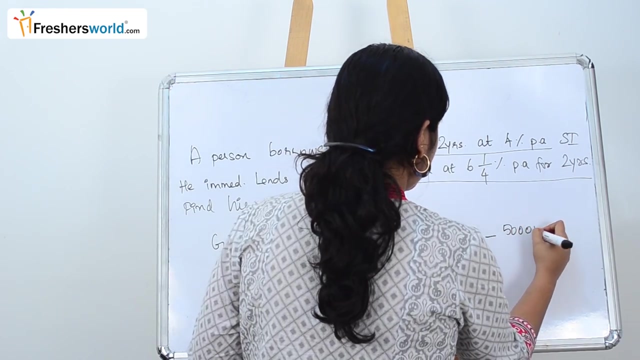 So we know the principal amount is 5000.. Number of years is 2 years and the rate is 6. 1 by 4 can be returned as 25 by 4 by 100, minus minus again PNR by 100. so 5000 into number of years is 2, into rate is 4 divided by 100. 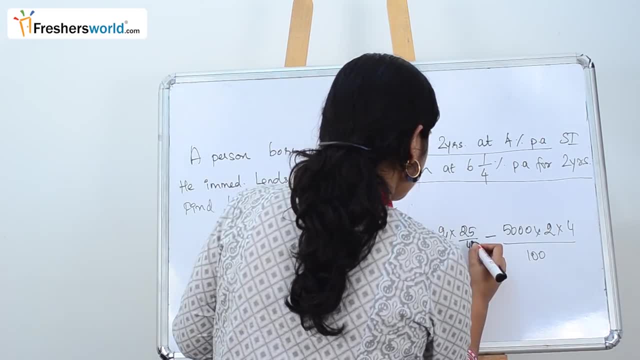 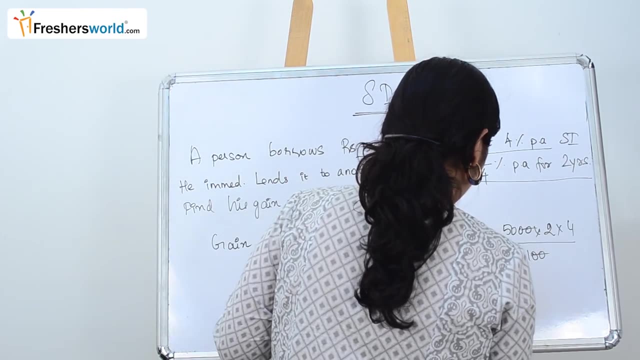 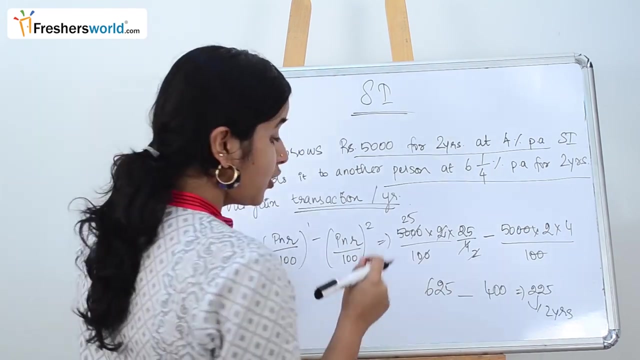 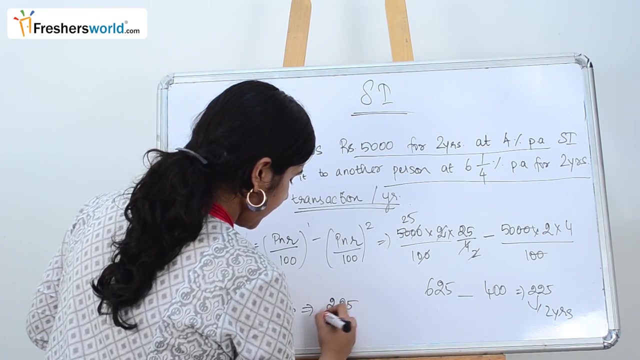 So let's solve this: Cancel 225 become 625, minus 8400 become 225.. So this is the gain value that he has attained for 2 years. So in order to find the gain transaction per year, which is nothing, but we know it for 2 years, is 225 divided by 2, which is 112.5 rupees. 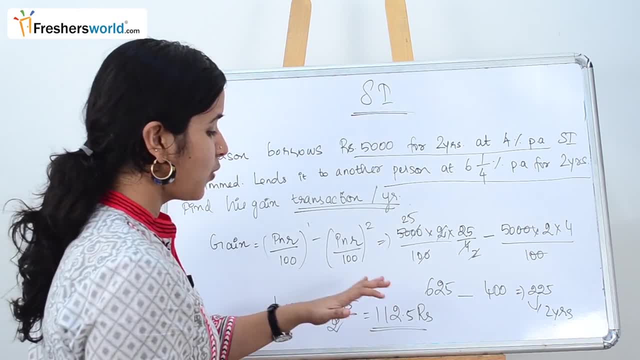 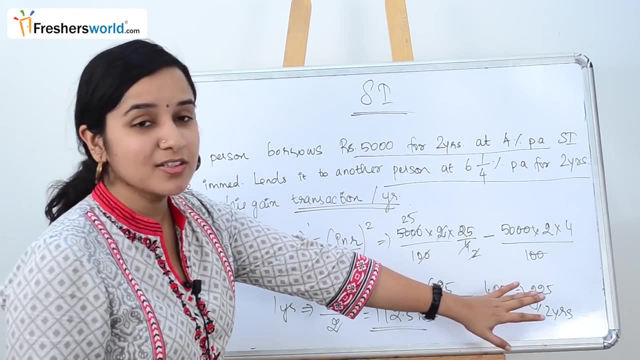 So the gain transaction per year is nothing but 112.5 rupees. So the basically, the mistake that lot of people make is that they will find the value to 225 rupees and stop it here, and you will know that in the option there will be 225.. But read the question again. they. 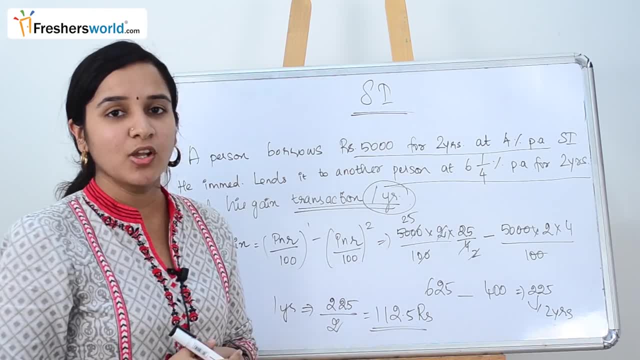 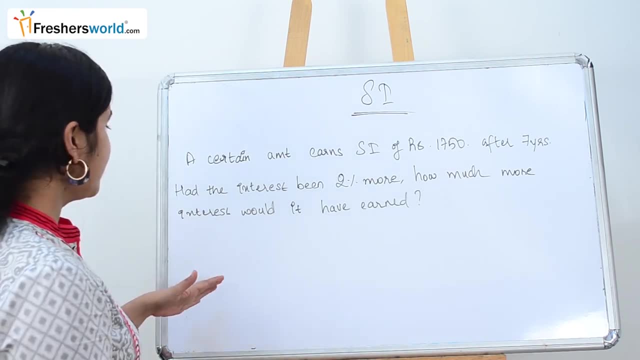 are asking it per year, So you have to find it only for 1 year. Let's solve it for another question. So the next question is: a certain amount earns simple interest, of rupees 1750.. After 7 years, had the interest been 2 person more, how much? 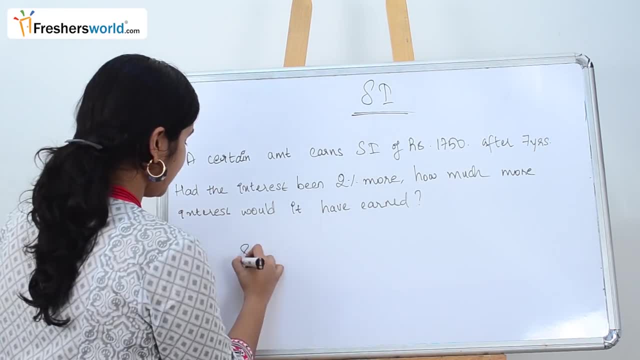 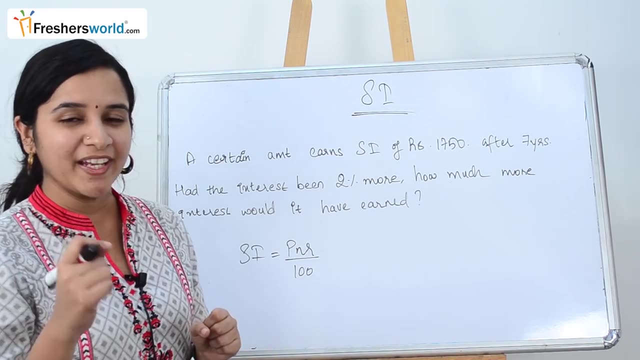 more interest it would have earned. So in order to find the simple interest, we know simple interest is equal to PNR by 100.. So at least 3 variable must be known in order to find the fourth variable Here if you see that the principle is missing. So if the 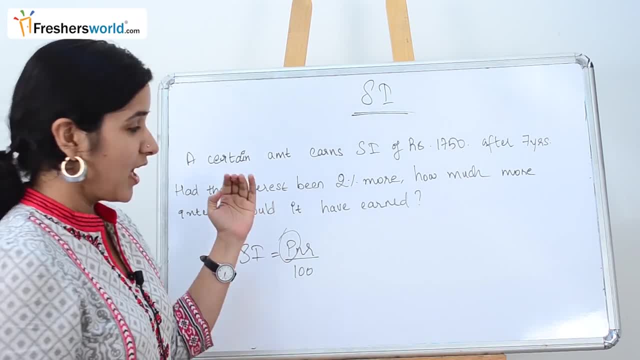 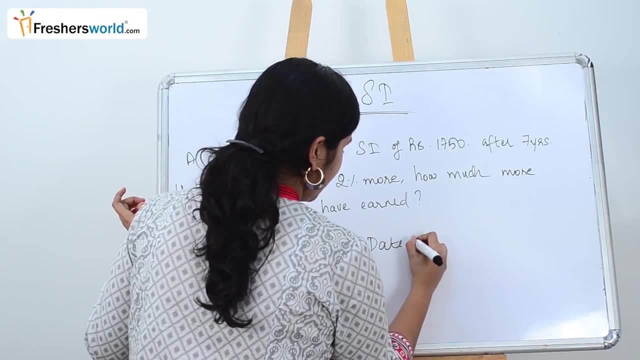 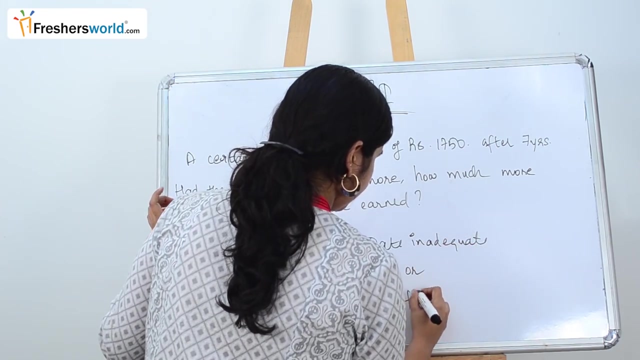 principle is not there, we won't be able to find the accumulated value for the number of years that they have given. so here the answer is nothing but data is inadequate or insufficient. but in order to confuse you, there will be another three, four option, which were where the 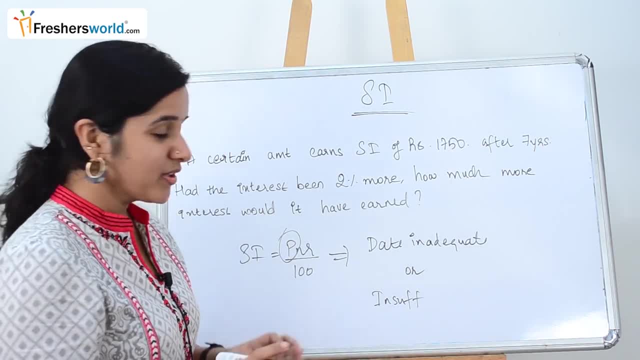 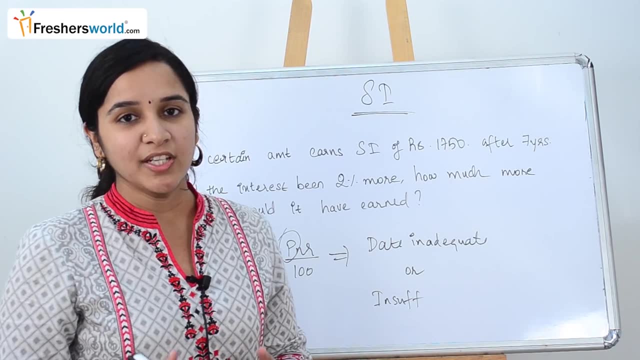 answer is given. but once you know the concept better, you know that without the principle you won't be able to find the simple interest. so that's very clear to you directly. you can select the option data inadequate. in today's video we dealt with the different types of. 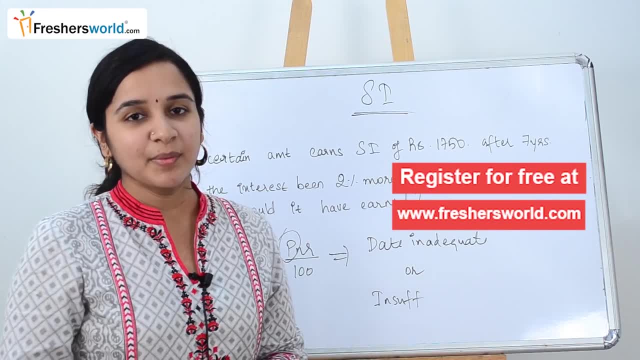 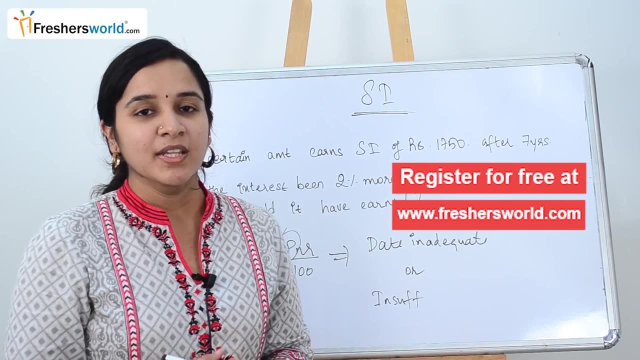 problems which you might face in the simple interest type of sums. in the upcoming videos we will be dealing much tougher problems in simple interest and we will also have compound interest as a part of our aptitude. so if you're a person who is looking for a job, kindly. 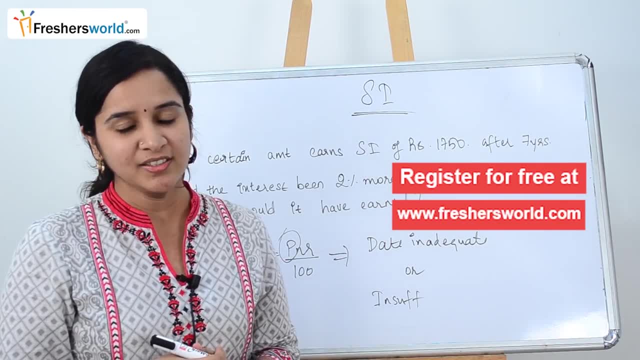 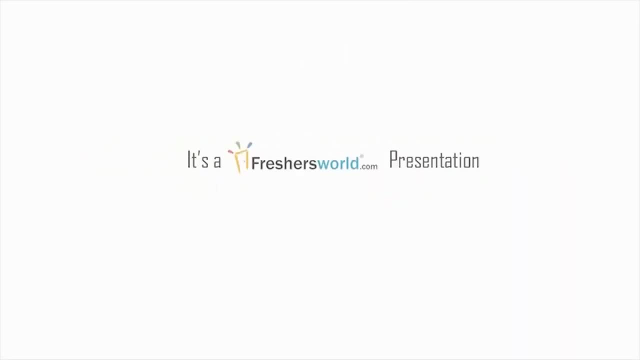 register in our freshersworldcom. like this video, subscribe to our channel. thank you you.